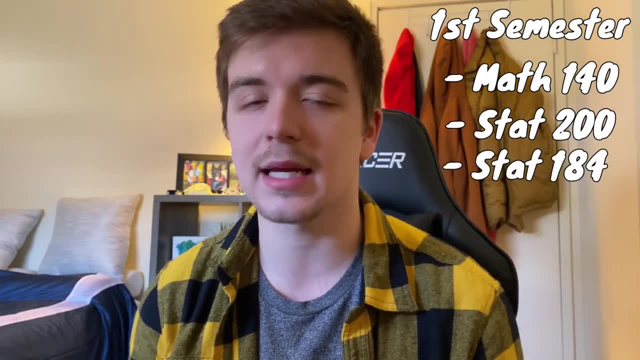 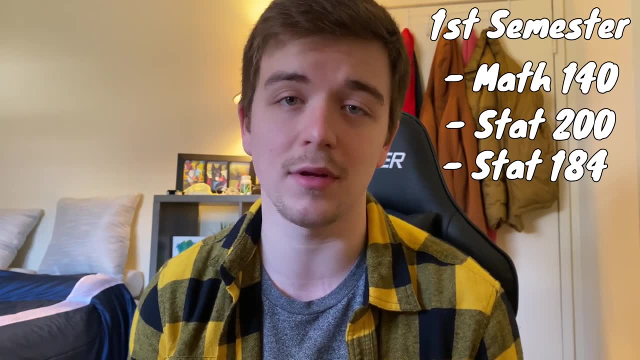 that everybody has to take pretty much at Penn State, And then you're also going to be taking Stat 184, which is called an introduction to R. Now, R is a programming language that you can use for a bunch of different things, but it's often used in academia for studying statistics. 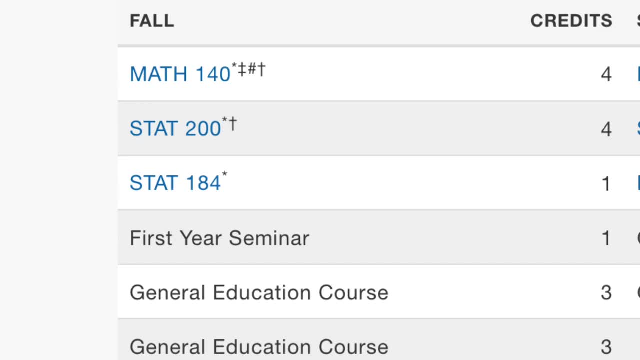 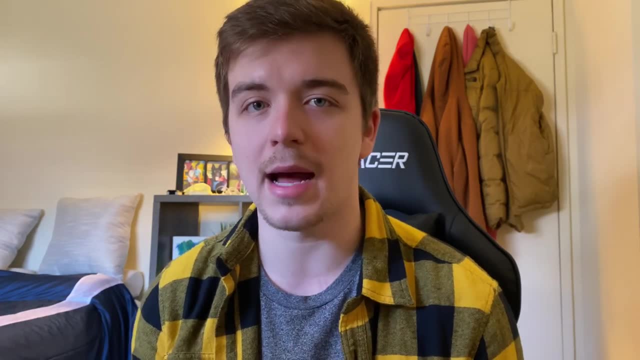 Now, on top of these three classes, you're also going to be taking some gen eds on top of it, so keep that in mind. But as far as those three prescribed classes, in my experience if you are familiar with math and if, especially, if you're taking pre-calc or calc in high school, 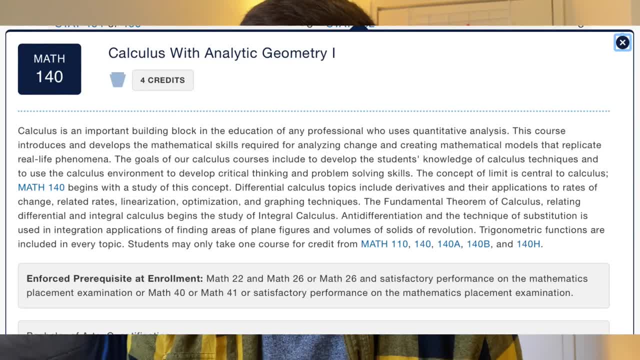 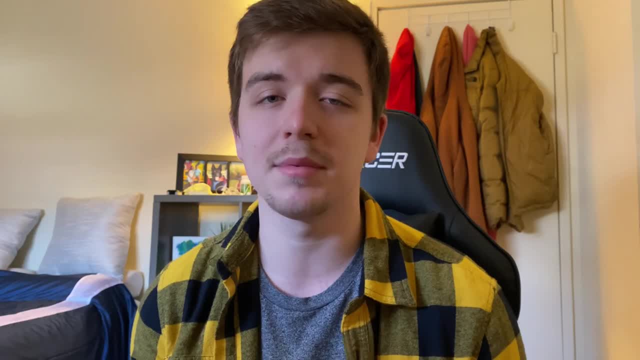 then Calculus 1 isn't going to be the hardest thing in the world. It's definitely a new experience if you haven't taken it in college or if you haven't had experience with calculus at all. I would definitely keep up to date on your mathematics, especially pre-calc, if you plan. 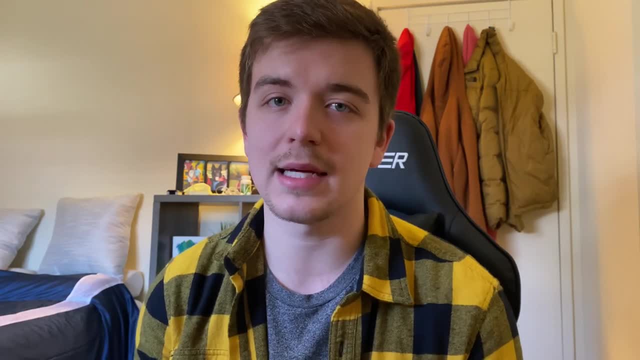 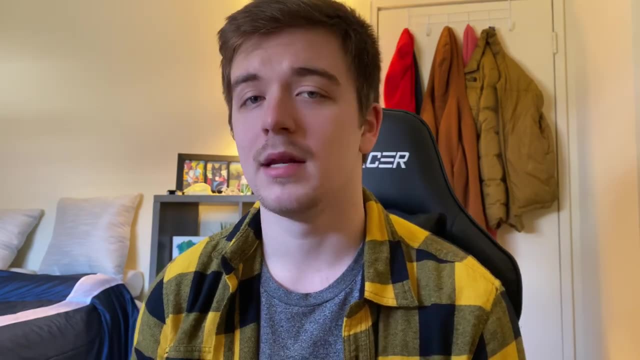 on taking this class. And of course this isn't going to be the only calculus class you take, because a lot to do with statistics is all based on calculus, so you're really going to have to have a strong grounding in mathematics. Now the second prescribed course. that was Stat 200 for the first. 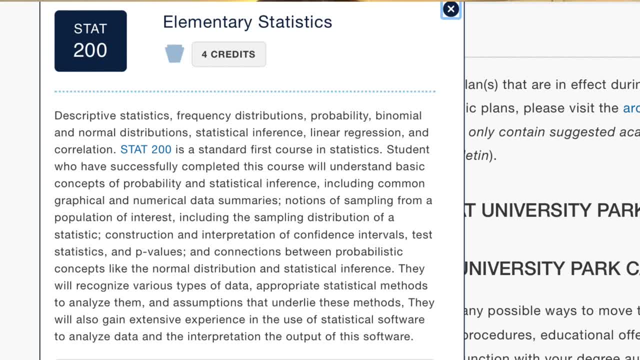 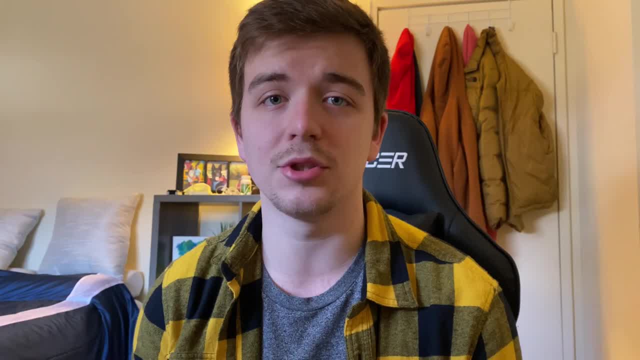 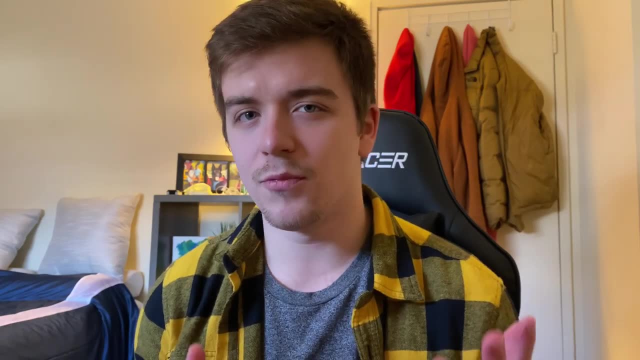 semester. this introduction to stats class is a really basic understanding of statistics. You're going to go over things like mean median mode. You're going to go over things like the normal distribution and some of the properties, Maybe some basic hypothesis testing and t distributions. Just rather simple stuff in. 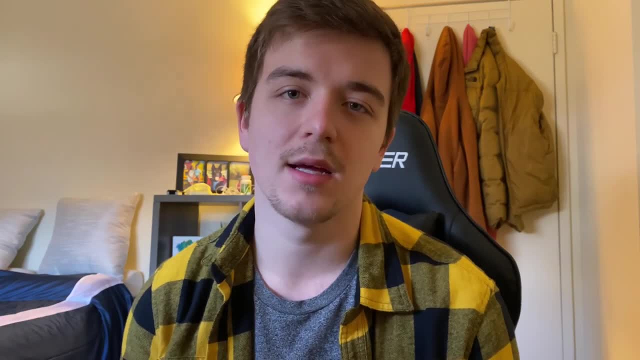 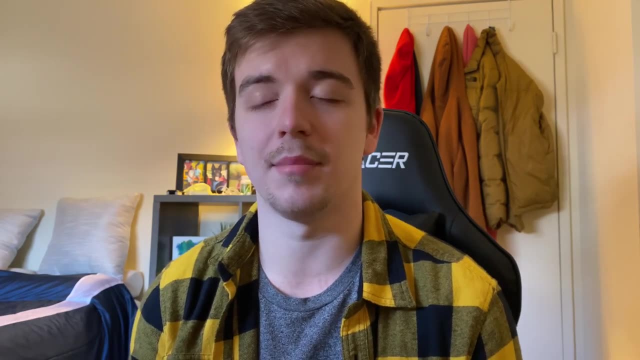 the statistics domain, but you're really going to want to pay attention to this class because it sets the precedent for the rest of your entire time at school. I wish I would have paid a little bit more attention in it, but for me it was kind of just a class that was thrown into a bunch of 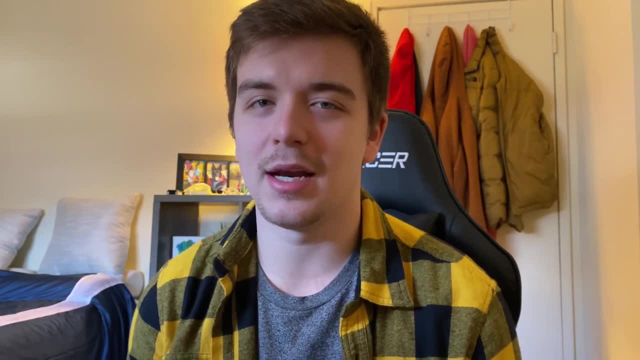 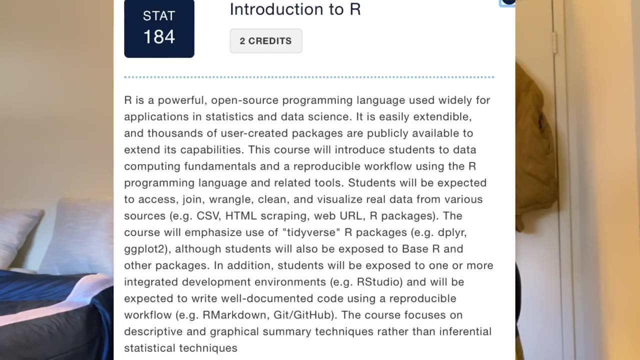 other hard classes with me, So I didn't really pay too much attention and it wasn't too hard to get through. but I definitely wish I would have paid attention and so I could have more solid grounding in the programming language of R. And now, finally, Stat 184, which is the last prescribed course for 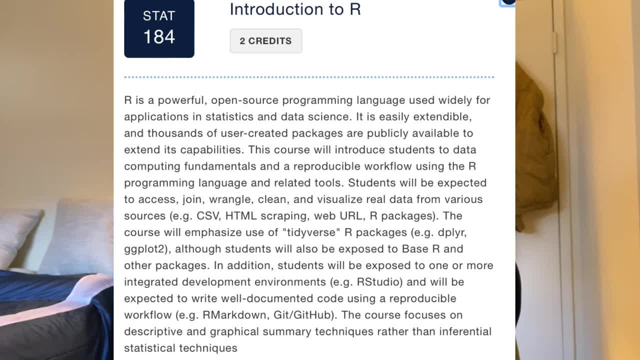 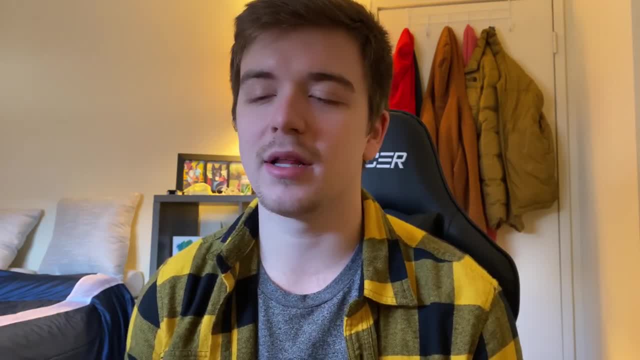 your first semester. I personally didn't take this in my first semester. I didn't take it till about my sixth semester, but definitely would have been helpful to take it before some of my other classes. So in Stat 184 you're going to learn some basic R techniques to manipulate data sets and analyze. 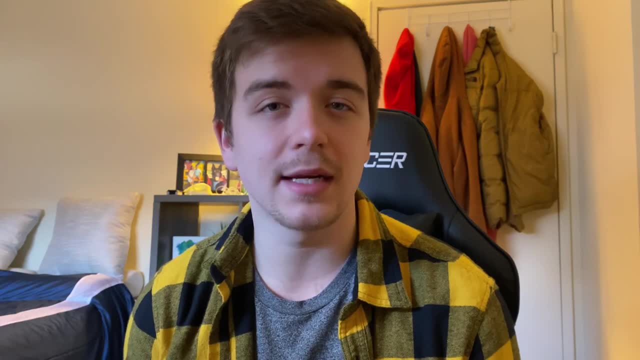 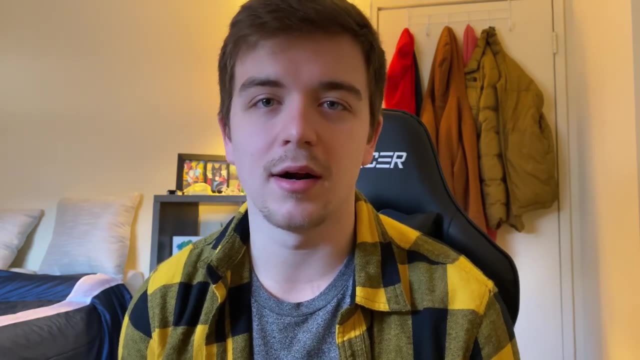 them in different ways. For me this was actually a really fun class. It wasn't too much as far as difficulty, but it was a great grounding in the programming language of R and it set me up for the future of my statistics career. So I've used the concepts I've learned in that class a lot. 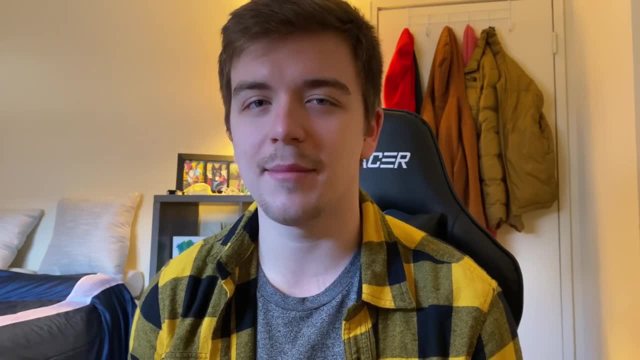 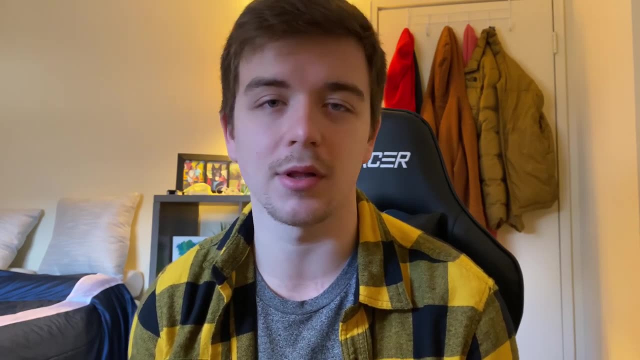 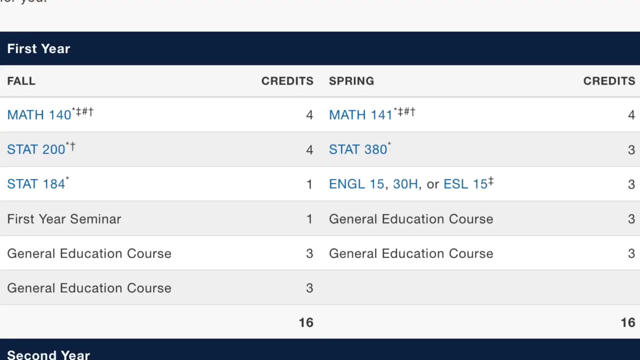 especially over the past year or so. But for this first semester I'm going to give it a difficulty score of around a six. It's really not too intense in terms of workload or in difficulty, so I think it's a great start into the statistics major. Now I'm only going to go over the first year of a Penn. 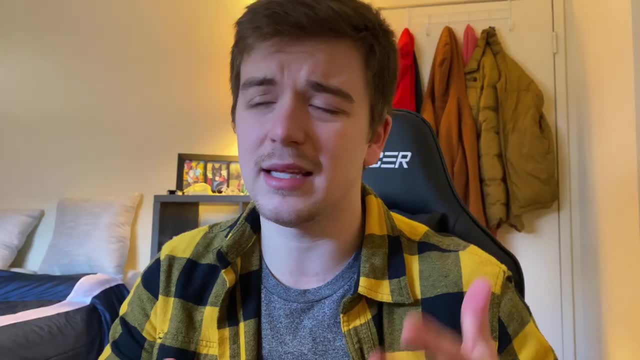 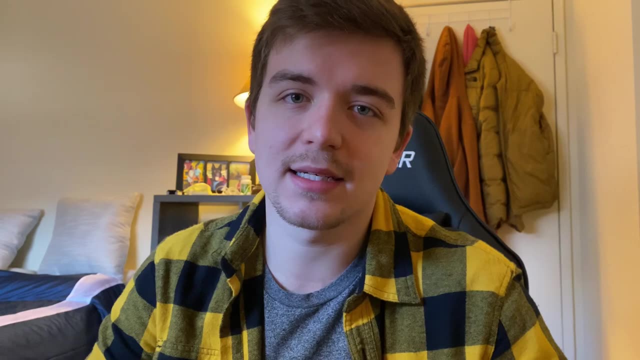 State statistics student, at least in this video. so if you want to see the entire statistics major at Penn State, let me know down in the comments below And I'll see you in the next video. But in your second semester as a statistics student, the only prescribed courses that are related to statistics are Calculus 2 and Stat 380. 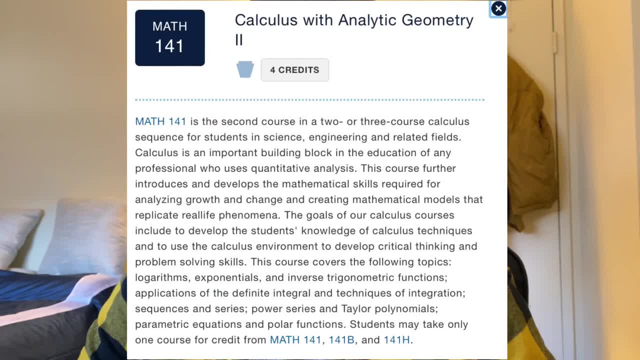 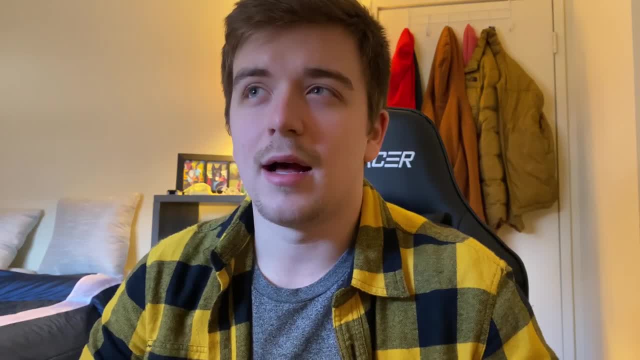 Now in Calculus 2, you're building again on many of the concepts you learned in Calculus 1.. You're going to get into more integrals as well as more advanced derivative techniques. I don't remember too much else from that course, other than that it was a little bit more difficult. 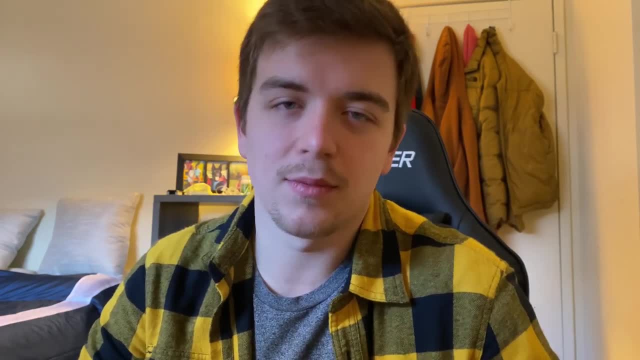 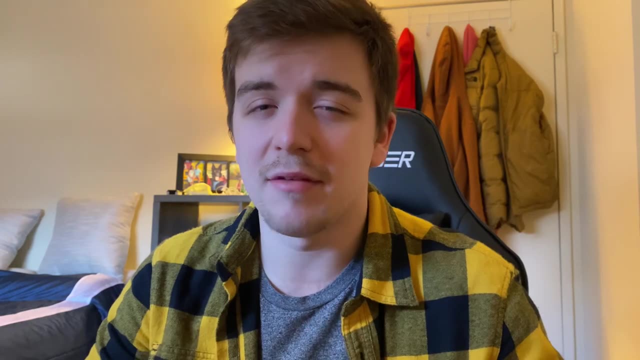 than Calculus 1.. But as long as you have a good basis in Calculus 1, I think you would be fine in this class. And one thing to note moving forward with a statistics degree is that you're going to be using a lot of math. So if you're not comfortable with it, 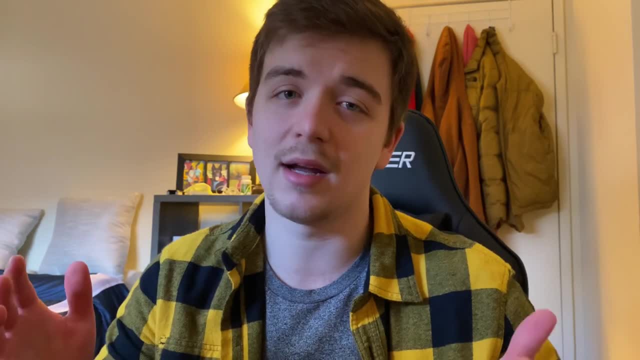 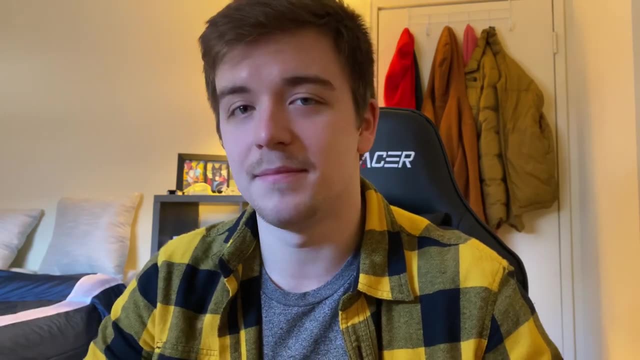 I would definitely consider practicing up, or maybe even not deciding with statistics, because that is a huge grounding in statistics and you're going to be using it all the time. And then I almost forgot one other concept in Calculus 2 that you go over. that is also very 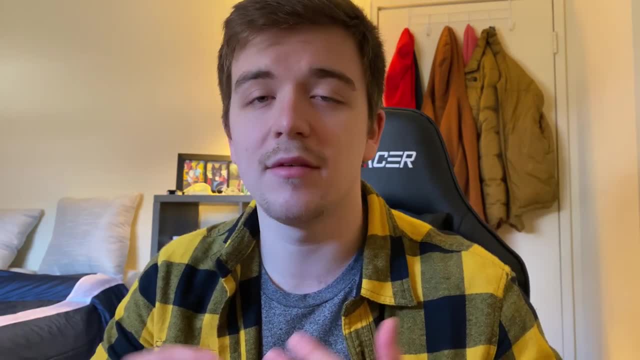 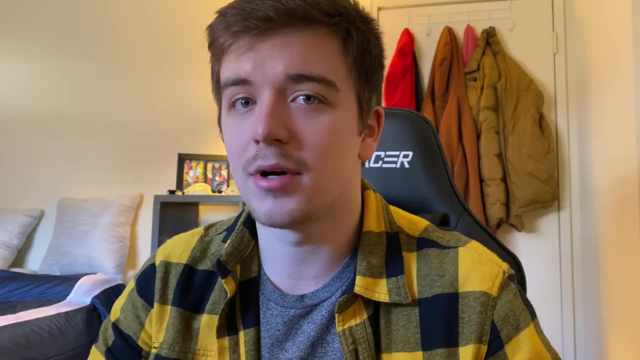 important is you're going to go over the idea of Taylor series and infinite series. This is another important statistics and you'll get into it a lot in probability later on in your statistics career. So keep that in mind as well. Now, the second prescribed course is going to be Stat 380. 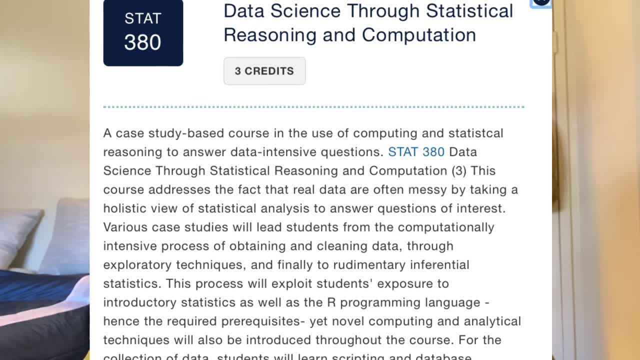 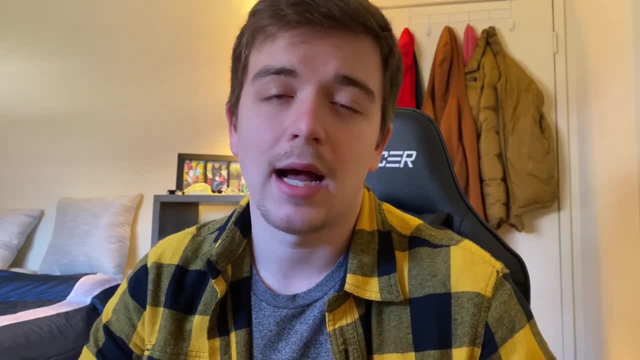 for your second semester. Now, even though it's prescribed into your second semester, I'm taking it right now as a senior, So you can kind of take these classes out of order. I wouldn't advise it. It definitely would make more sense to take it in the order that they give you. But the name. 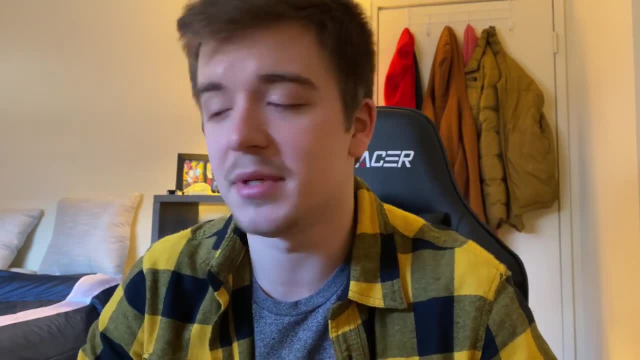 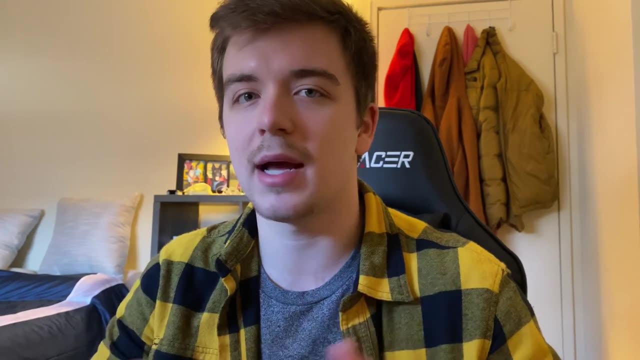 of this class is Data Science through Statistical Reasoning in Computation. So in this class you're going to learn a lot of what you learned in Stat 184, which was the introduction to our class, and you're learning to apply it to a data science application. So what you're doing here is you're